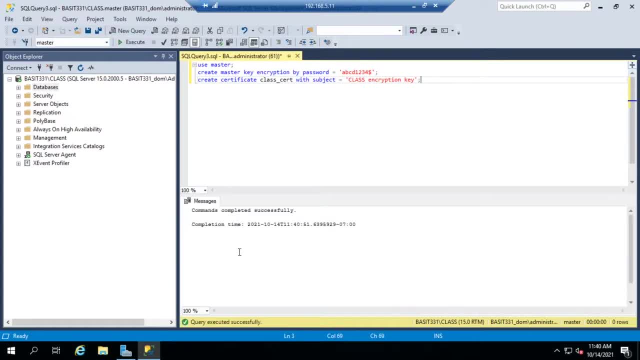 And execute. okay, so that will create the certificate for us. now you're definitely going to want to back up the certificate. we can, um, we have that backup if we don't do that, because this is going to back up the database and it's going to, or it's going to, encrypt the database, and even when we 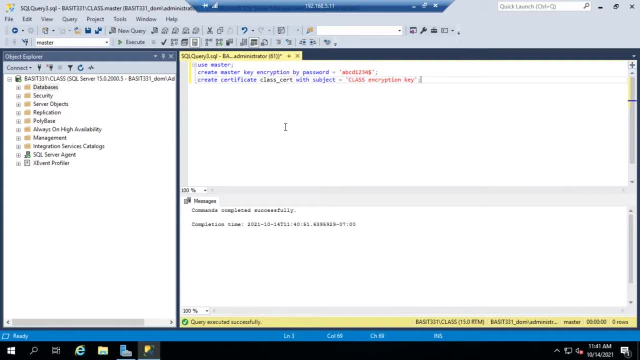 back up the database. it's going to be in that encrypted state. so if something ever goes wrong and we lose this uh certificate or we need to restore this database somewhere else, without that certificate we kind of have a problem, like we can't get to the data. so we need to make sure. 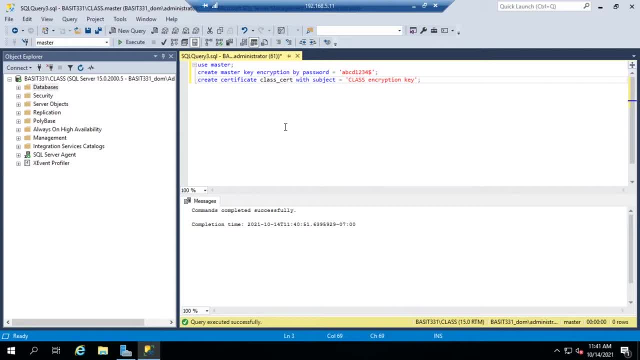 we back that up now. i could continue on and do the rest of this in uh transact sql, and we'd use the adventure works database and then we'd create the database encryption and set encryption to on. we can also do that here in the gooey, however, so i'm going to show you how to do that. 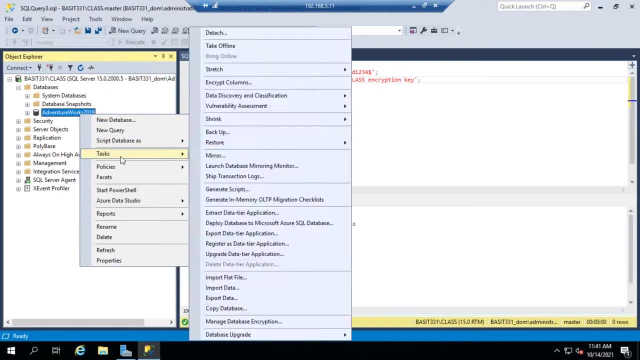 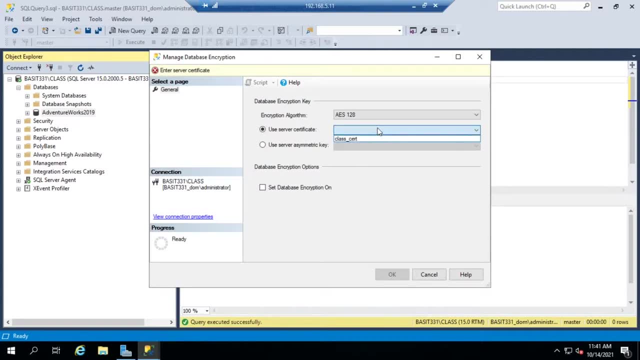 there i'm going to right click on adventure works and in tasks we're going to go to manage database encryption. so we've already used the certificate or we've created this certificate and we need that certificate so that we can use that here. you class certificate notice. 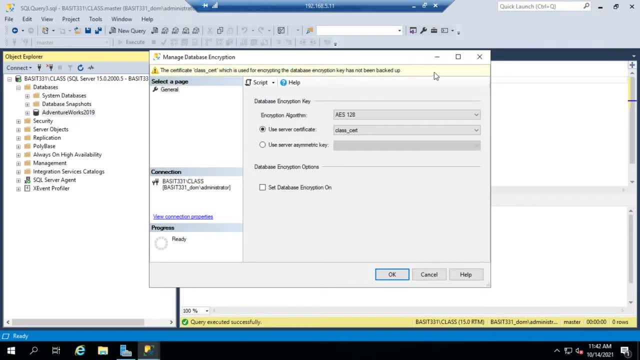 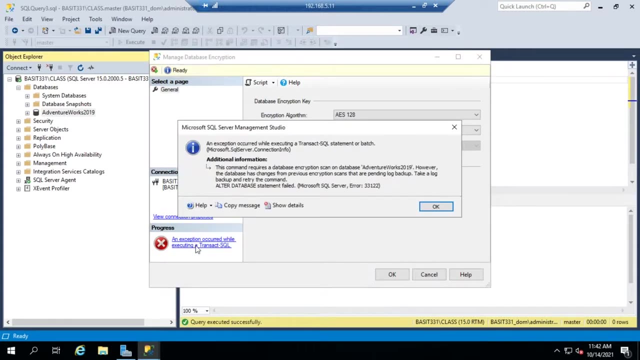 is going to warn us this hasn't been backed up yet. okay, fine, and then we're going to set database encryption to on and hit OK. now it's actually going to encrypt for us in the background, and we actually ran into an error here. ah, I was playing with it earlier and it 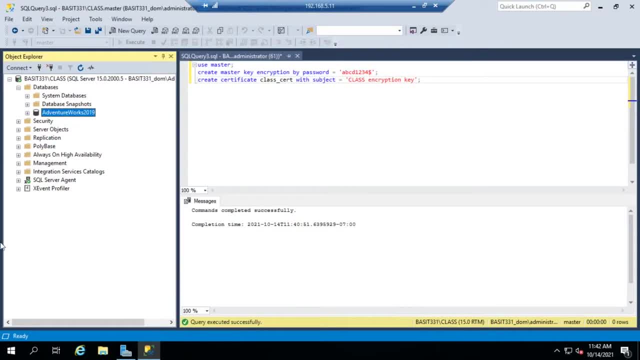 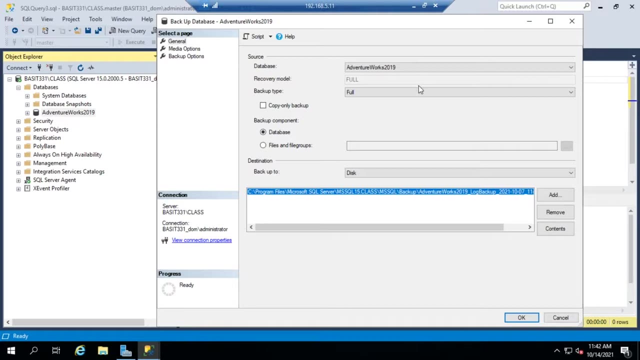 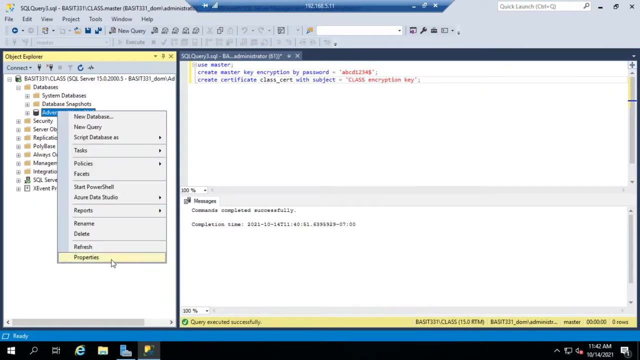 needs a log back up real quick. so slight detour here: right-click- we're going to do a backup. go to tabs, asks back up and I'm just gonna back up the log transaction log back up and okay, we'll just do a real quick log back up and that should clear it and allow us to do this. so right-click and tasks. 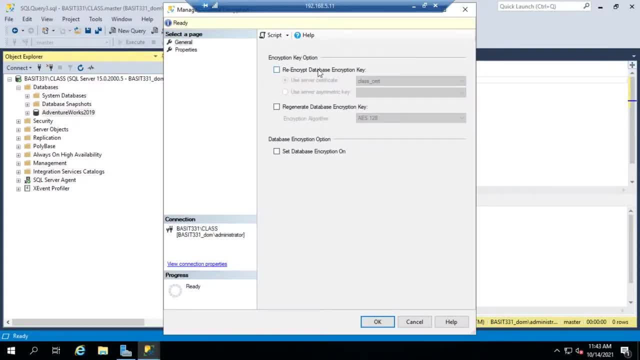 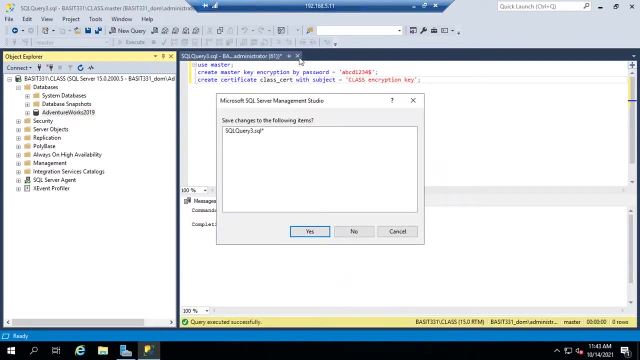 and manage database encryption. we're going to re-encrypt using the certificate and said database encryption encryption to on and hit OK. okay, there we go. that actually worked the way we wanted it to. okay, just a real quick thing we had to fix there. now that does our encryption. the encryption happens in the background you. 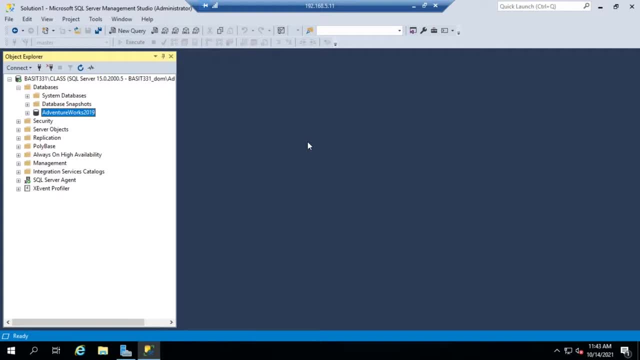 can continue to use the database. but they're going to be a few challenges, like kind of what you just saw, where I tried to do something and wouldn't let me because I needed to do a backup real quick. so some things are going to be tied up while we're doing this encryption, so you may want to schedule. 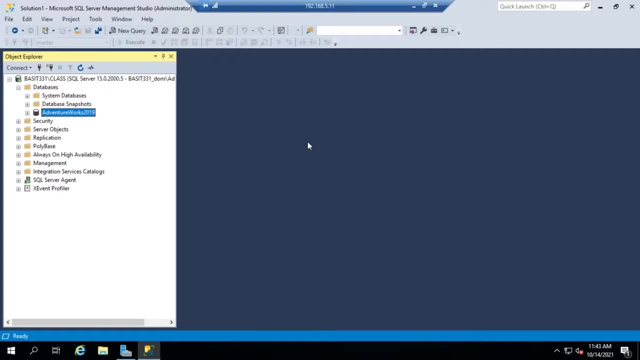 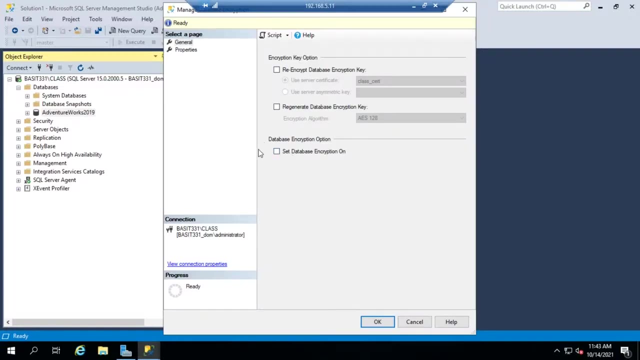 this to happen off hours or do it early on now. this is a small database so it should happen pretty quickly now. if I ever want to turn that off, I just go to right-click tasks- manage database encryption and then I'm going to set day or uncheck that set database encryption, to awe or uncheck that set database. 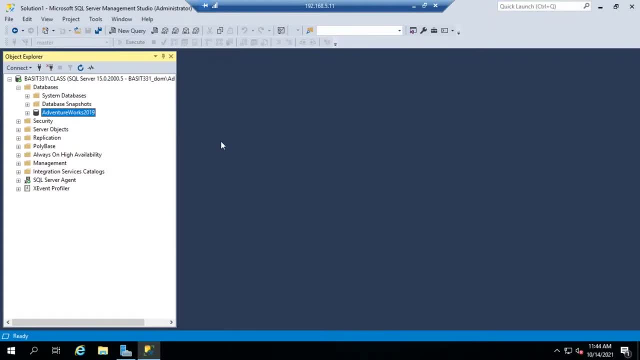 encryption to on and that'll turn it off for me and that will then decrypt that database. okay, that's how I can encrypt the entire database and I can also encrypt individual columns. I'm going to expand this out. there's a couple of different ways we can do this, and they're basically just different ways of. 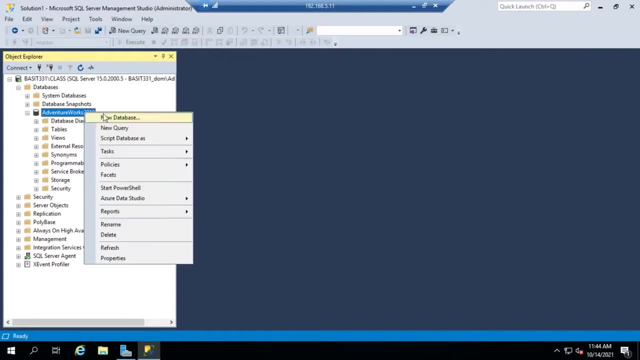 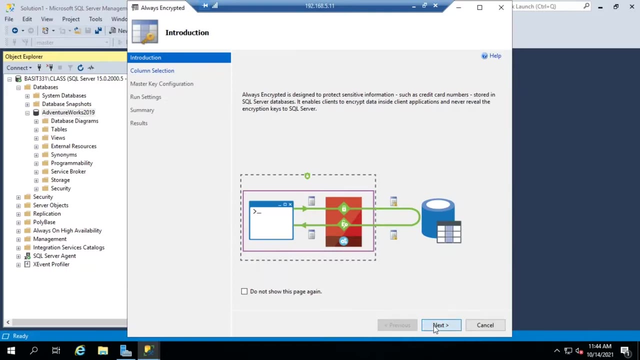 getting to the same point. so we can right-click, go to tasks and choose encrypt columns, and this is only going to do specific columns now, because I'm doing this at the database level. what's going to happen is, when I go to column selection, it's going to show me every single column in the 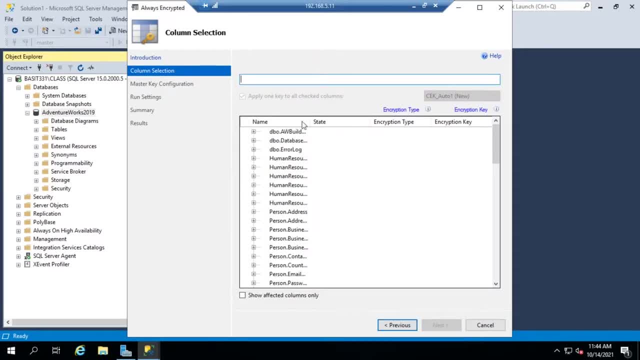 database, and then I need to go through, expand this so we can see this a little bit better. and then I would go through every single one of them, select- see which one did I want- not that I wanted- the pay history and I want to encrypt the pay rate and then I can go to the employee and I can. 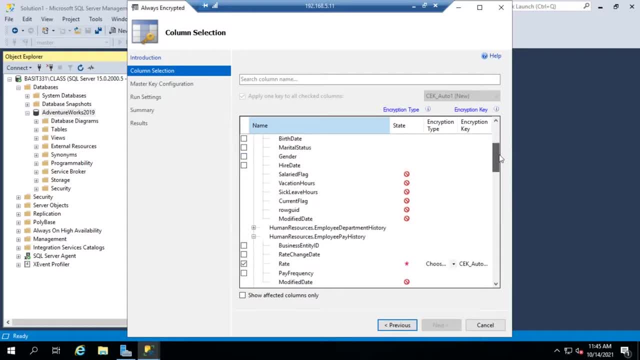 choose whatever it is that I want to encrypt here. notice, by the way, some things can't be encrypted depending on the type of data it is, so I can go column by column and choose everything in my entire database that I want encrypted. now, to me this is a little challenge. you can do a search here, so let's do rate and this. 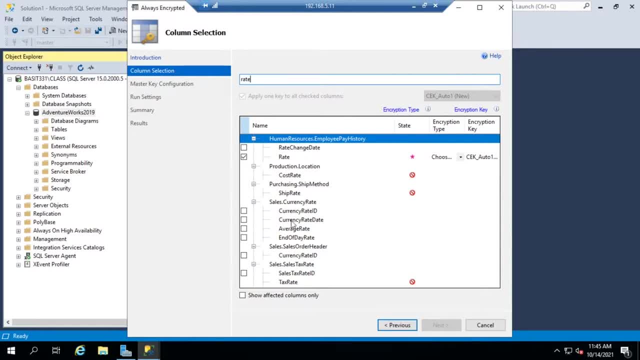 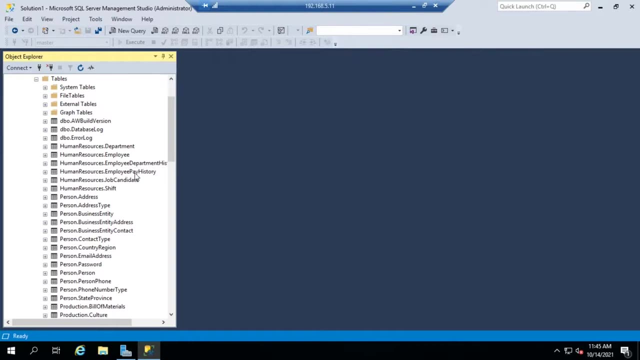 will show me all of my rates that I can, or all of my columns that have the word rate. so that'll kind of help filter this down a little bit. now another option is to go to the actual column itself. so I can go to tables and let's say I wanted to do the entire table or view the entire table. I. 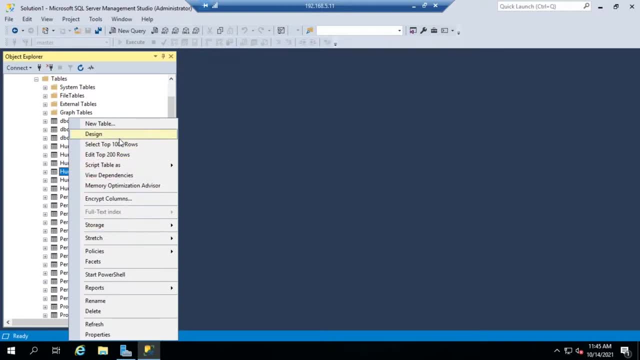 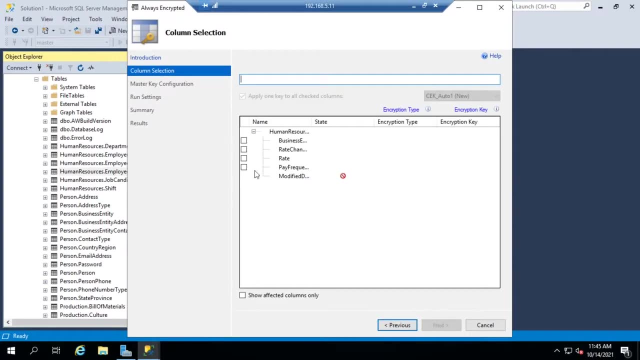 can right-click on pay history and go to. I just thought there it is- encrypt columns and this will take me to the same place, but now it's only showing me that one table. so if I don't want to sort through everything in the entire database, this might be an easier way to find it. another alternative is I can. 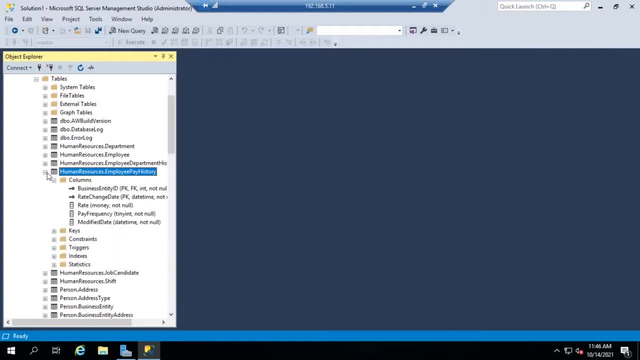 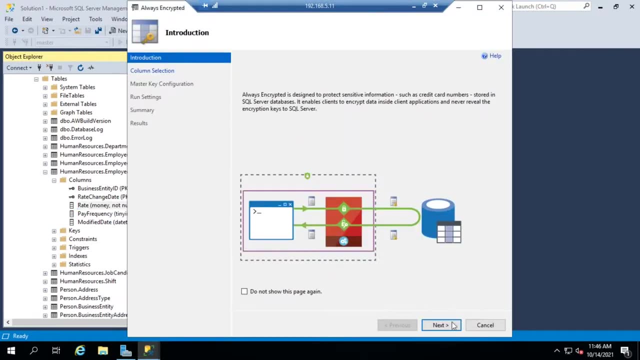 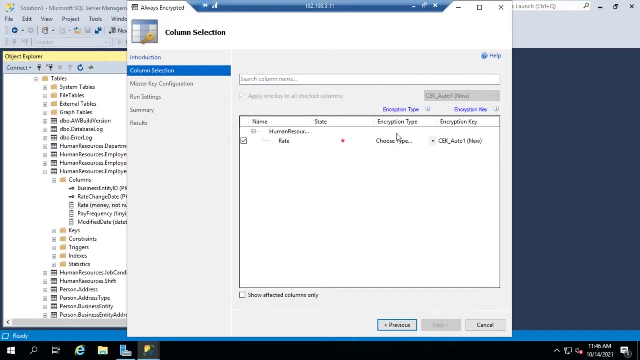 expand even farther and right-click just on that one column and go to encrypt column, and now when I go to column selection, it shows me just that one column. okay, regardless of what we do- I need to or how we find it, I need to choose type, and there are two different types of 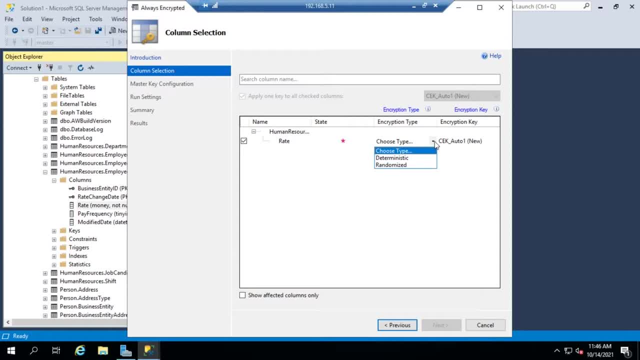 of encryption, there's deterministic and randomized. all right. deterministic means the same data will be encrypted the same way every single time, all right. so this is Ray column. so if I had, you know $25 an hour, that $25 will always be encrypted the same way and it will have the exact same ciphertext every time. 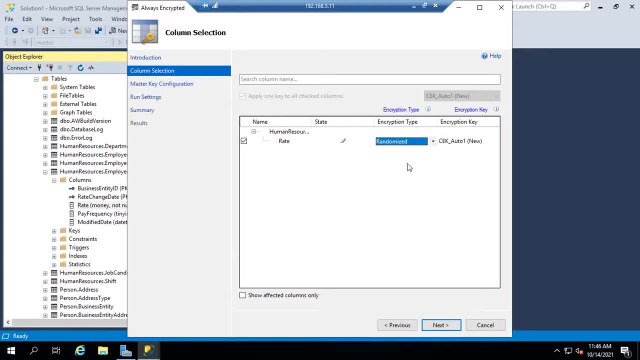 it's encrypted. now randomized is maybe a little bit more secure because it randomizes that encryption inherently to give me the date one, and so it doesn't look the same way every single time. I encrypt 25 one time and gives me one block of ciphertext and the 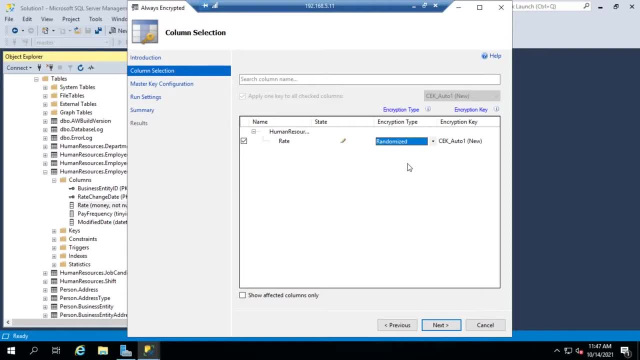 next time I do it might give me a completely different block of ciphertext. now the downside of that randomized encryption is there are certain operations we can do on it, so we can't Jawteam accept removing units to a control- blancum columns that are encrypted through that randomized method. if it was, 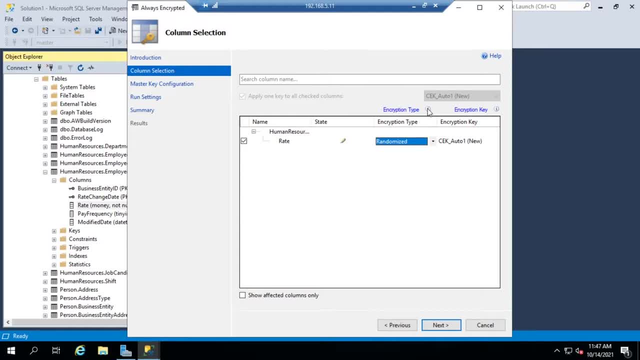 deterministic. we could not have that feature because we can't uncompress a. we could join, by the way, anytime you see this little, i click here to give me more information and notice here. it tells you kind of what we're talking about. randomized encryption is more secure. 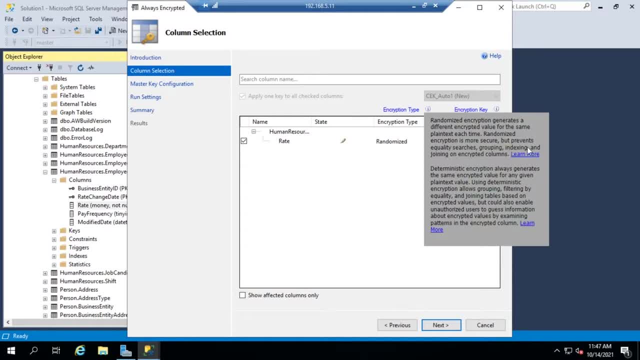 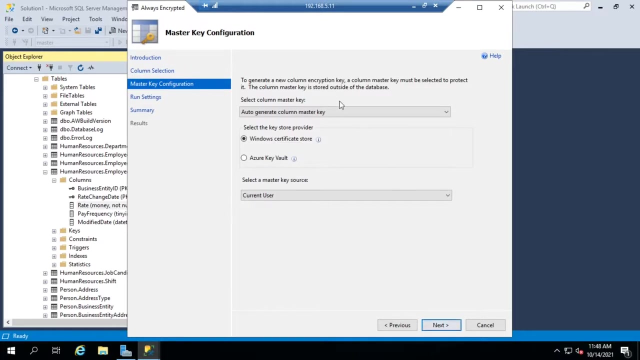 but it prevents equality searches, grouping, indexing and joining on the encrypted columns. deterministic always gives the same encrypted value for any given plain text value. so just we were talking about and then we can choose an encryption key or, because i haven't done this before, it will generate a new encryption key for me, so i click next and then we will auto generate. 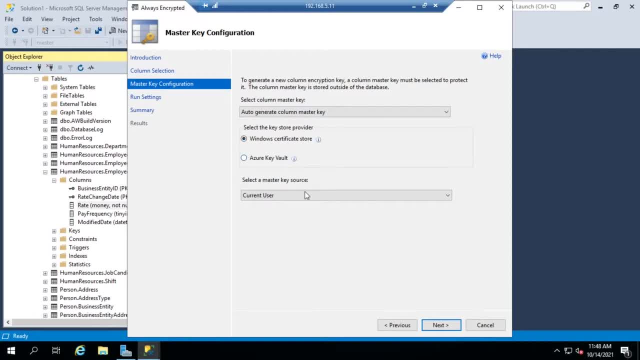 we select key store provider: either the windows certificate store, the azure, we can set the key source to be the current user or the local machine and then either we choose the key source or the local machine, generate a powershell script or do it now. the advantage of doing this powershell script is i can set it up. 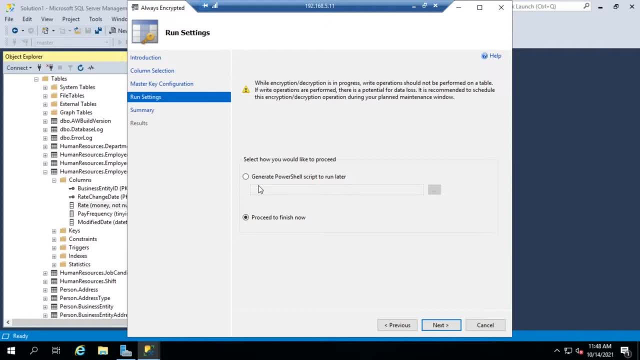 and then i can, you know, create all of my scripts that i want and say, alright, this encryption might be a little bit of a time consuming process, so i want this to happen later tonight when i'm not here. so i'm going to generate the scripts and have one of my junior admins just execute the. 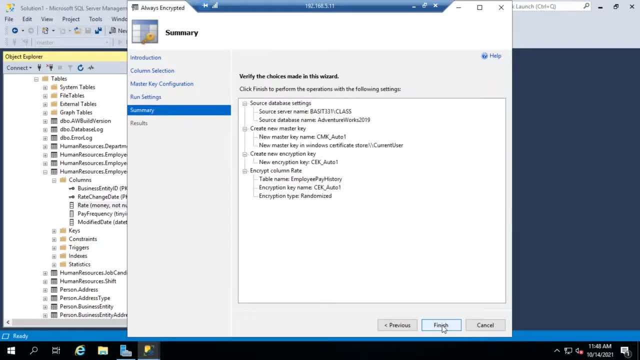 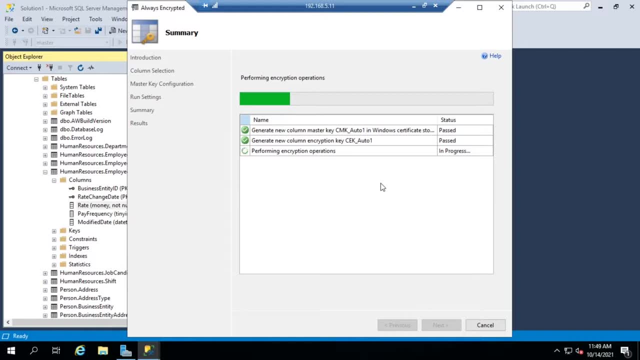 powershell scripts. alright, if i want to do it now, i just click proceed to finish now, and and finish, and that will start the encryption for me. ok, there we go. that is how we will set our encryption in our database, either for an entire database or for the. 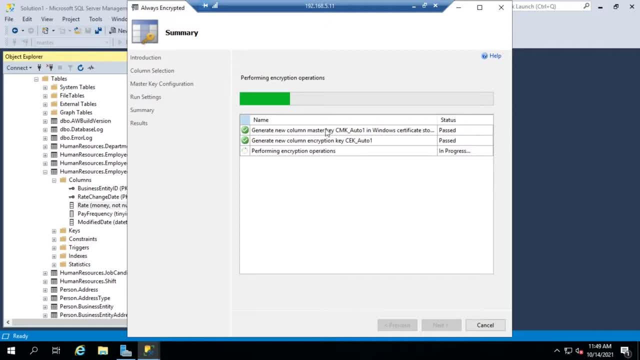 uh, specific columns now. remember i said this is going to take a little while. you can see its progress right here. encryption is a fairly intense operation, so i'm just gonna let it run and i'm not going to run it just so. its이�very intense operation, so i'm just gonna let it run and that's pretty much it. so encryption is a fairly intense operation, so i'm just gonna let it run and that's pretty much it. But now you know how to do it.